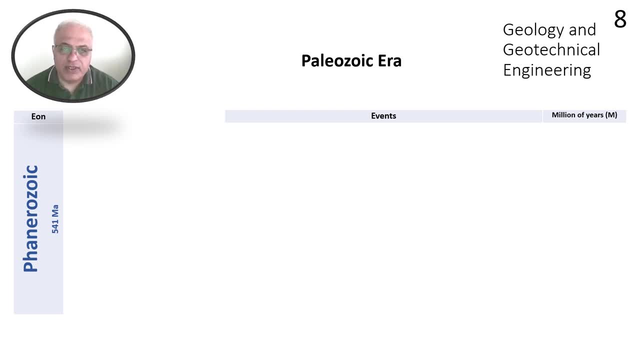 And the Paleozoic Eon is divided into three major eras. The lower part of it, called the Paleozoic Eon, is the time of the geological time scale. The lower part of it, called the Paleozoic Eon, is the time of the geological time scale. 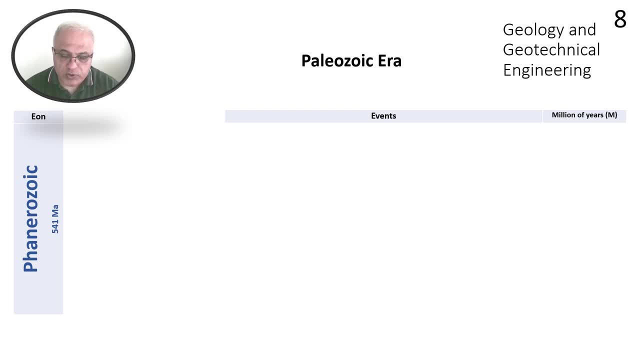 The Paleozoic Era, which we are going to deal with it in this presentation today, and in the middle of the Phanerozoic called the Mesozoic and the upper part of the Phanerozoic called the Cenozoic Era. The Paleozoic spans around 290 million years and divided into six major 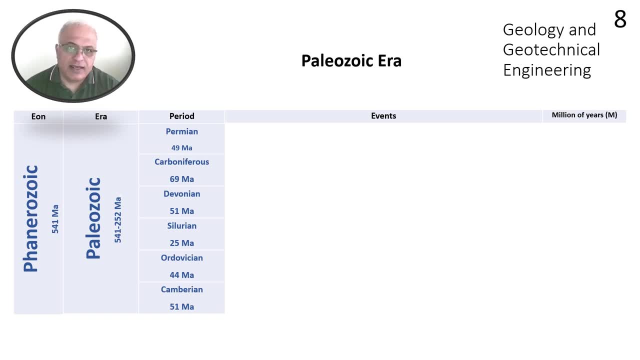 periods, according to the events and the catastrophes happen to the planet earth, starting from the cambrian. the cambrian spent around 51 million years and the major events in the cambrian is the domination of the multi-cells organisms, and especially the trilobites, and 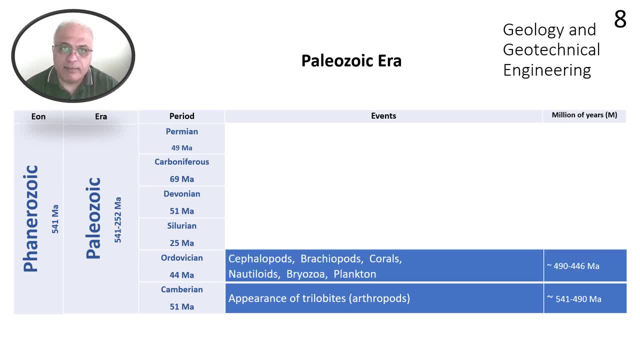 the ordovician, the multi-cells organism, dominated the oceans of the earth, and examples of this domination is the uh, cephalopoids and the, the, the brachiopoids and corals and nautiloids, and also the borzoa and plankton. 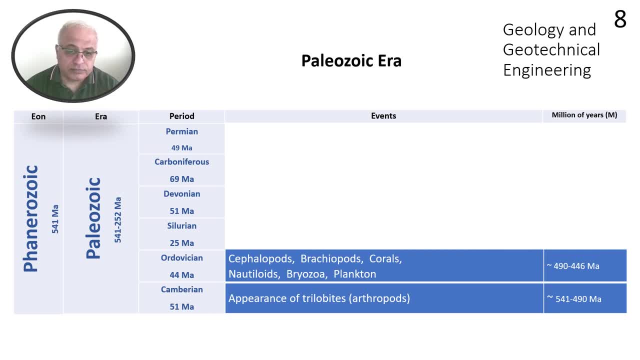 organism: the, the, the, the silurian. the silurian has spent around 25 million years, is the shortest period of the paleozoic era, and during the silurian many metroids strike the and impact the earth surface, and these changed the climatic events of the earth. 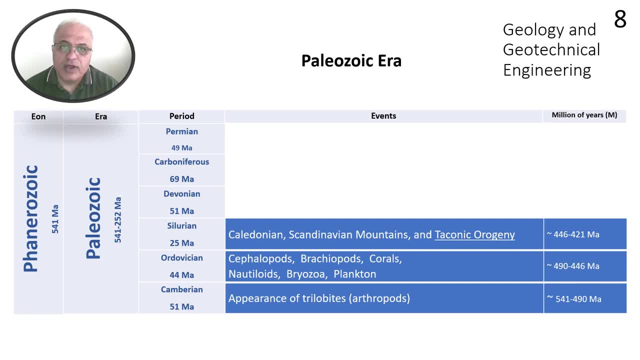 and, and, and and there are. there are also around eight stages in the silurian. there were the climatic change, climatic changes being recorded, uh in the rock formation belong to this period of the earth history: the devonian, the. the devonian period characterized by uh spreading and domination. 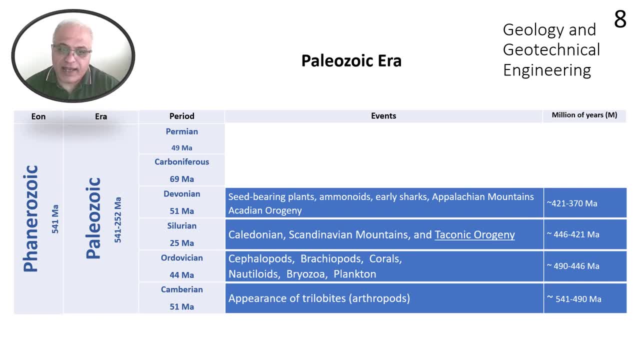 so there's gonna be one culture too, of the seed bearing plants and trees and also the ammo it's: the early sharks have been found in the oceans of the uh devonian and also opportunities. uh many origin has been recorded uh in this uh period of time and the the the main origin is is the appalachian mountain change building and also the. 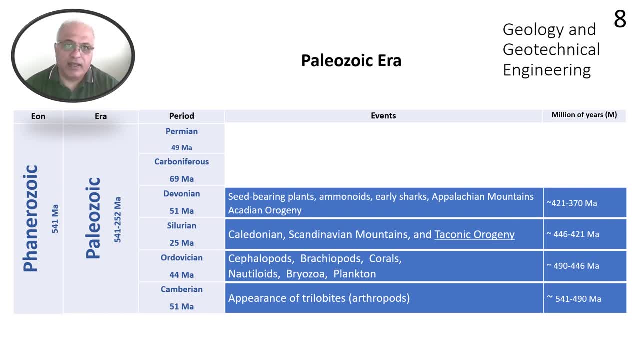 and also in Asia, the Oral and Himalayan mountain chains being also built up during this period of time. The Carboniferous, characterized by domination of the amphibians and forests. and this period of time ended in fact, or separated from the period. 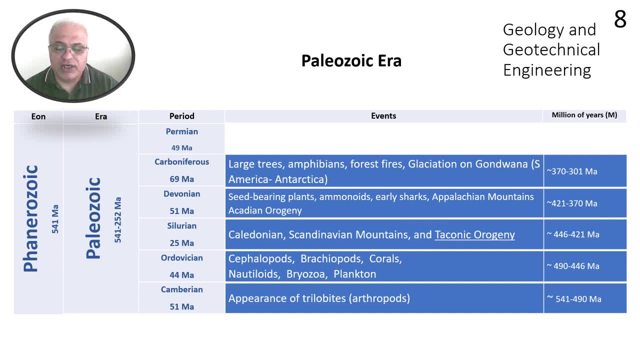 After that, by a huge glaciation covered all the planet Earth. due to the climatic changes that happened to the planet Earth during this period of time, The Permian characterized by the existence of the great continent, Pangea and also the end of the Carboniferous Glaciation. 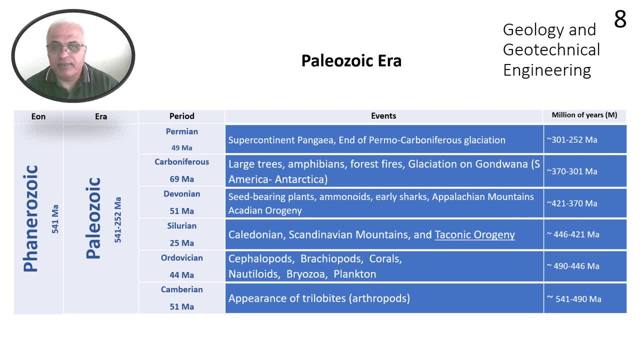 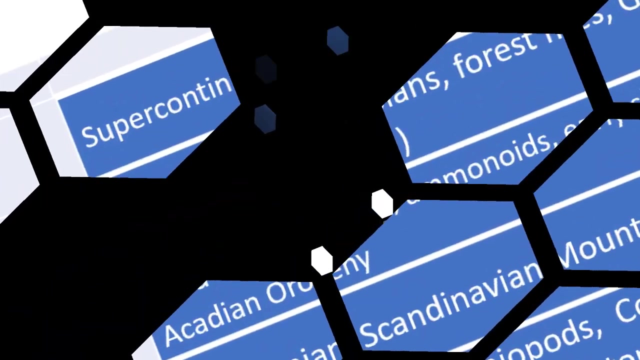 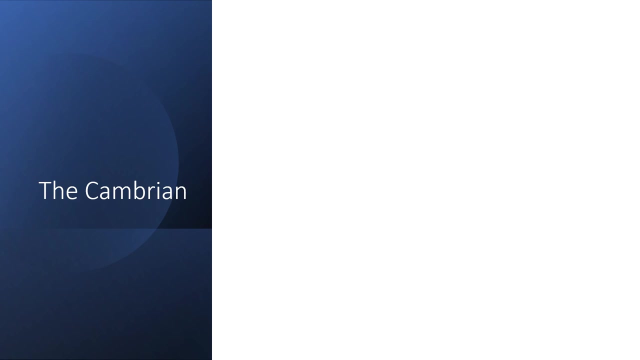 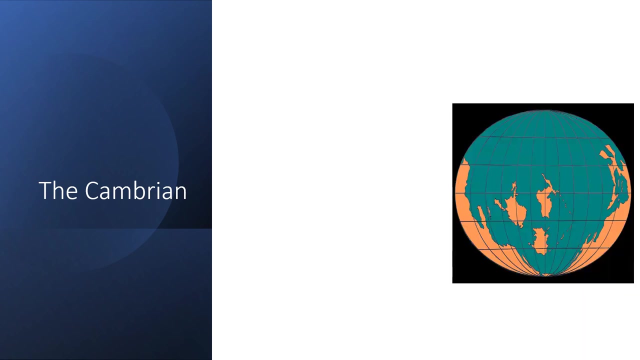 The following is a brief presentation for each of these periods of the Paleozoic Era as an attempt to understand the development in the history of our planet Earth. Now, as mentioned before, the Cambrian period span around 51 million years and the Earth shows up, like shown here in this Earth map of the Cambrian. 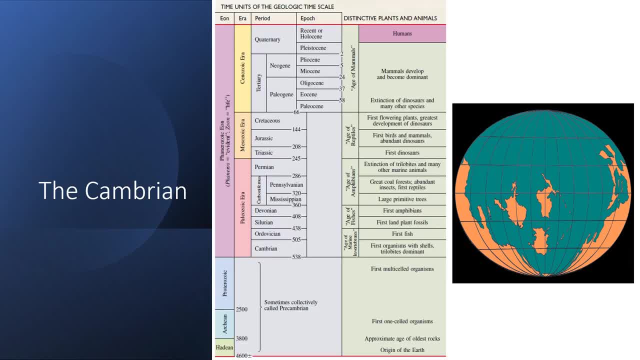 and the position of the Cambrian in the geological timescale is shown here at the lower part of the Paleozoic Era In general, the life in the pre-Cambrian time, or the Proterozoic unit, the late part of the Proterozoic era. 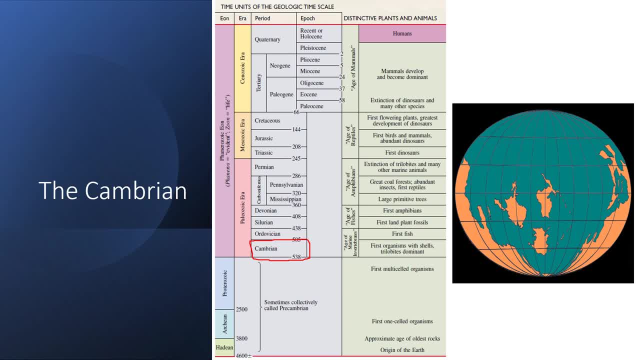 the Proterozoic eons calls. of course, the pre-Cambrian was dominated by unicellular or simple one-cell organism. In the Cambrian, the food chain of the organism based on algae and a huge modification happened to the life or to the marine life. 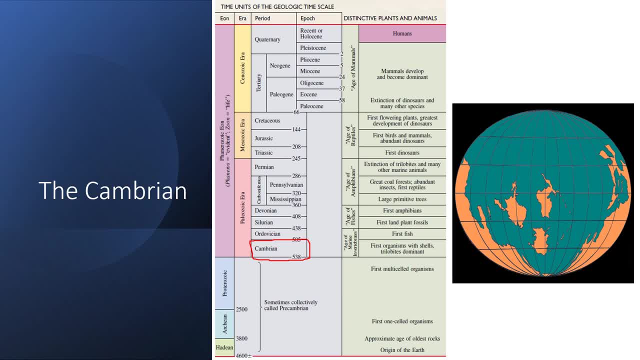 of the Earth. in the Earth's oceans, The multicellular organisms dominated the oceans of the Cambrian. Through this period of the Earth history, a rapid diversification of life forms happened, and known as the Cambrian life explosion event. This event spans around 25 million years. 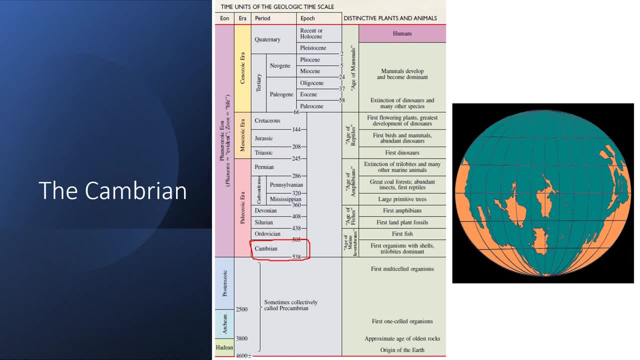 and left spores in the sediment and rocks belong to this period, Evidence found in South Stake Formation in Wales and in the one-kilometre-thick motomorphic rocks- sandstone mudstones of Hollywood. The Earth's climate was cold during the early stages of the Cambrian period. 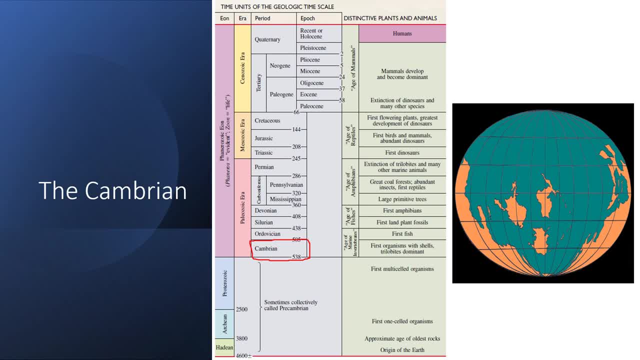 because the continent Gondwana situated near to the south pole of the planet Earth. The average temperature recorded in the rock formation of the Cambrian was about 7 degrees centigrade higher than our day's average temperature of the planet Earth. 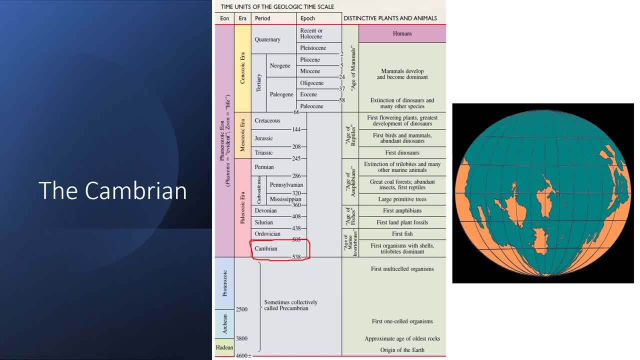 The Earth's pools were covered by ice In the Cambrian. the Earth was recovering from the global glaciation of the late pre-Cambrian or the late period of the Proterozoic Eon In the end of the Cambrian. 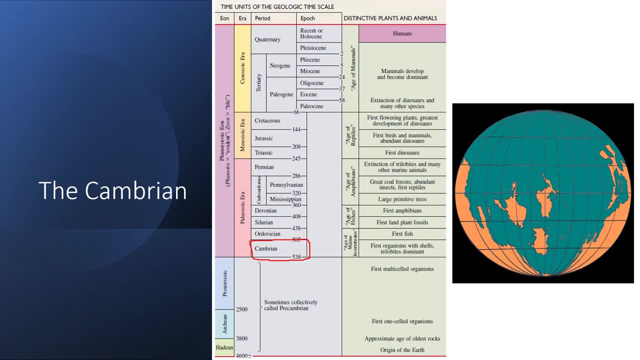 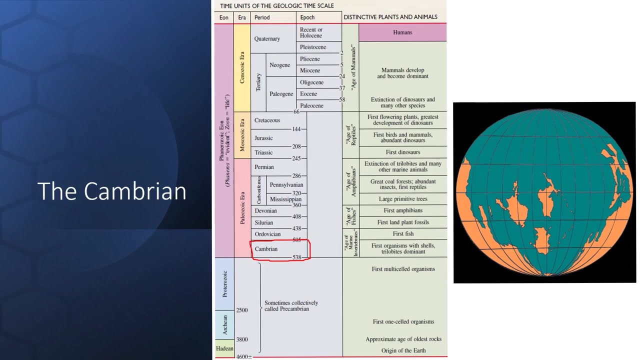 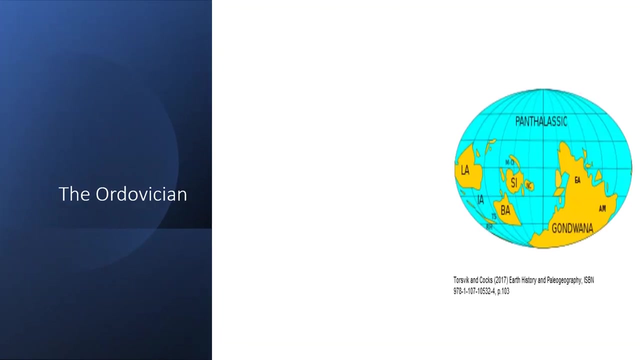 the glaciation receded, disappeared and the sea level rose by ice, fresh water, reducing the salinity and adding more dissolved oxygen to the oceans of the Cambrian. The Ordovician period. the Earth shows up as shown here in this image. 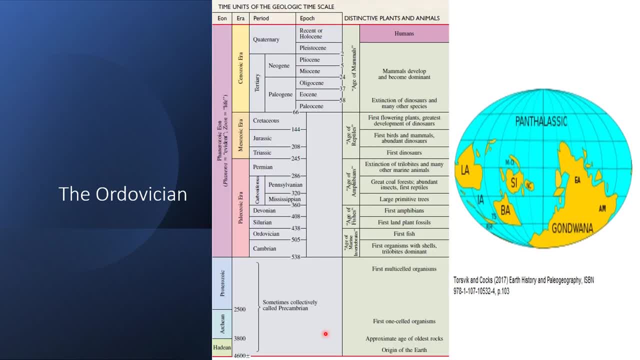 and the position of the Ordovician is shown here in the geological time scale, which is a part of the Paleozoic era. The Ordovician separated from the Cambrian by a notable change in fauna and documented in the Walsh, a lower Paleozoic bedding system. 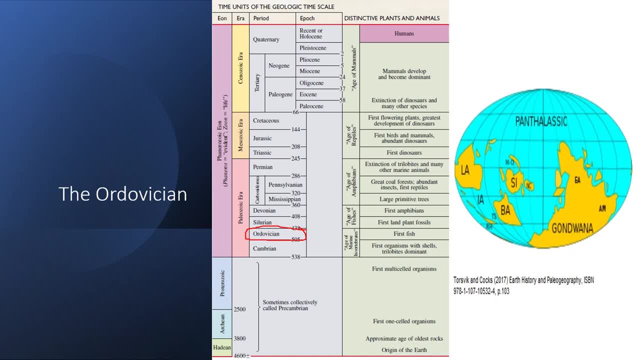 The bio-diversification event, increased by fish species, dominated the period, this period, and dominated the oceans of the Ordovician. The Ordovician recognized by a strike of meteoroids much more than our days. Therefore, the Ordovician included 20 stages of climatic changes. 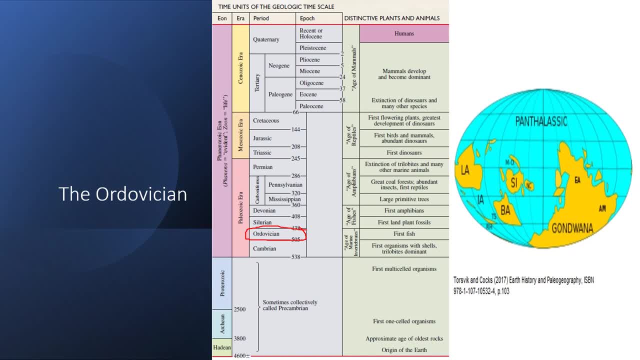 The Ordovician seas dominated by mineral calcite, which is inorganic marine precipitated mineral combined with carbonite, composing the oolitic limestone which later became a suitable oil reservoir, The biogenic type of the calcite called the aragonite mineral. 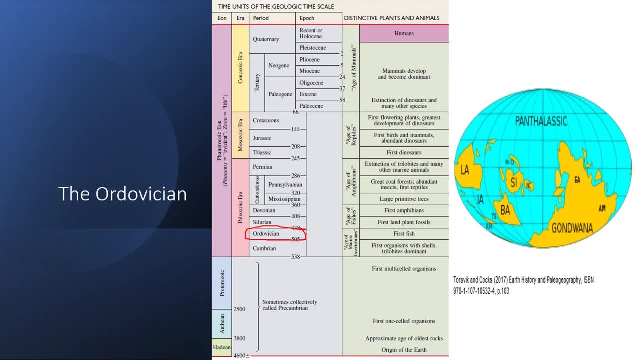 this type of mineral composed the shells of the mollusks and dissolved again in the seas of the Ordovicians. after the death of this organism, The climatic climate of the early Ordovician was very hot, but the late Ordovician 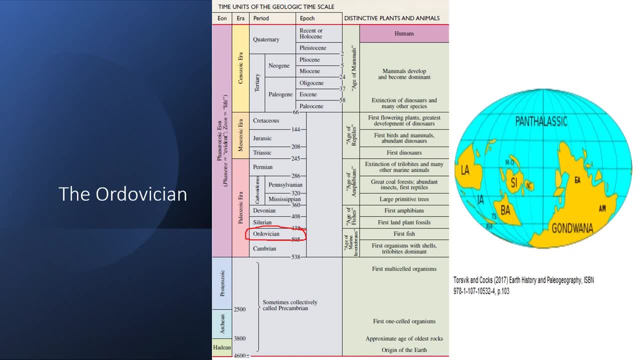 the climate became cold by glaciation intrusion of Hernetian glaciation. The sea level dropped down and more continents exposed to the weathering processes. The Ordovician end with one of the largest extinction event of the earth history. 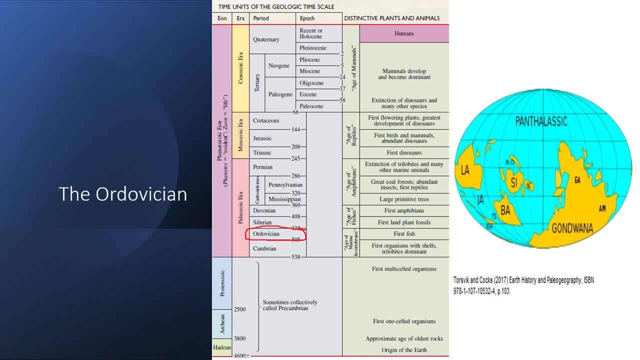 The other extinction events happened in Permian, the late Paleozoic era, to Triassic, which is a part of the Cenozoic era. The Ordovician extinction spanned around 3 million years and marked inconformity. 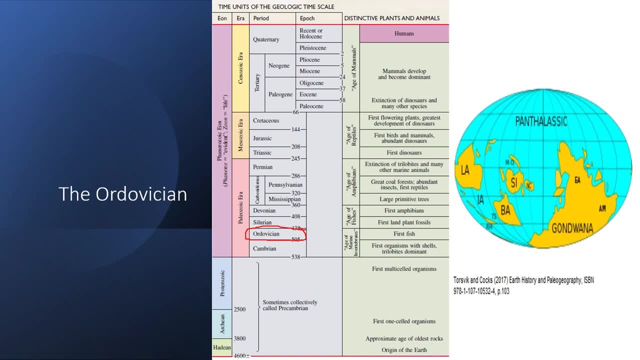 and beginning of a new period called the Silurian period. By the end of the Ordovician period, 49% of fauna were multi-celled and dominated: dominated by the Brachiopodes, the Porozoa. 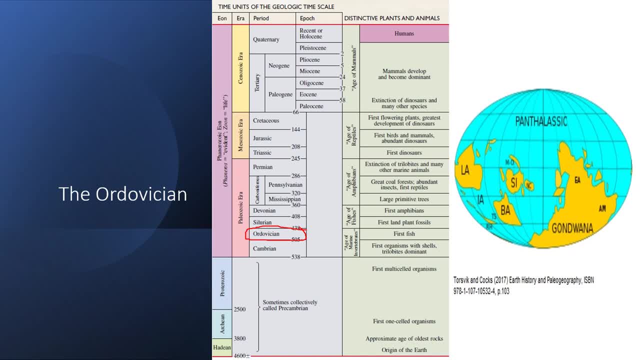 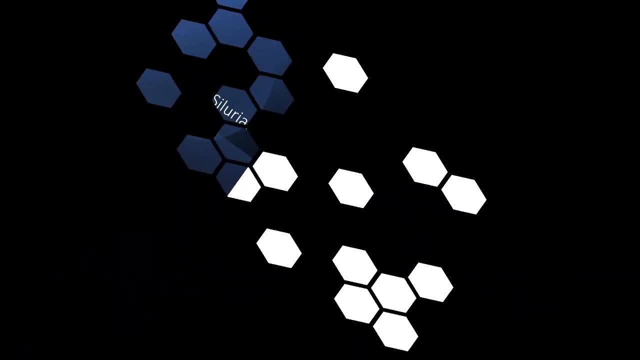 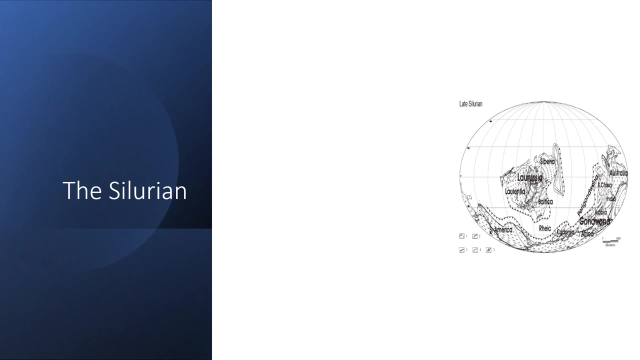 the Trilobites and the Graptolites, The Silurian period. the earth shows up as it is shown here in this image, and here we can have distinguish the continent of Americas and the the sea of. 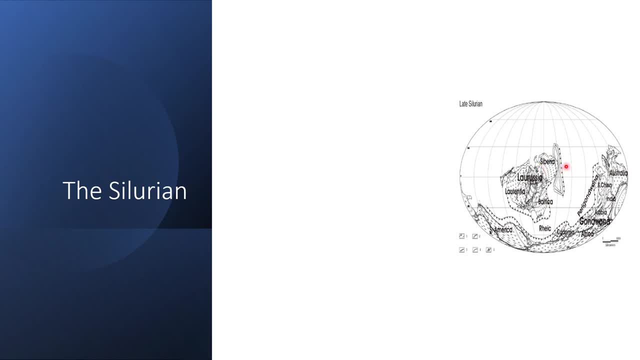 Ritik, and also the Siberian, the Laurasia, the Baltic area and also the India and Australia continents shown here. The image of this continent is the shown here is the subduction zones. 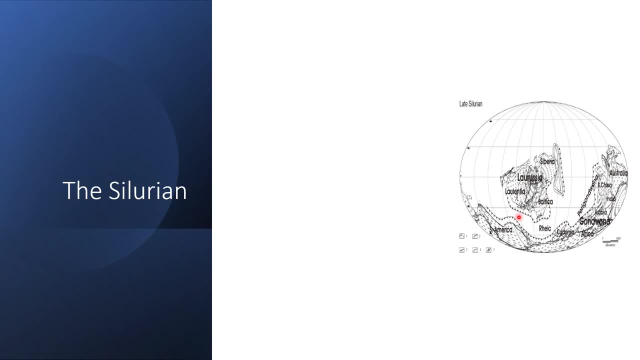 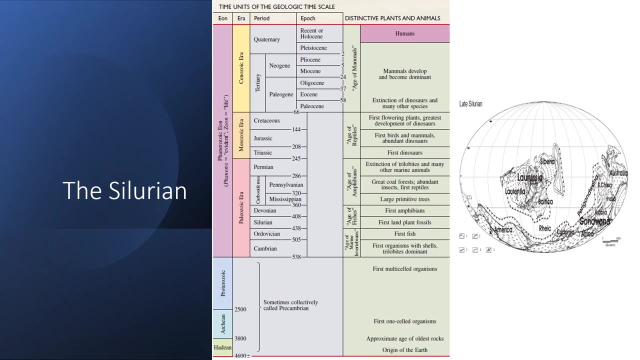 with the oceanic plates. The position of the Silurian is shown here in this geological timescale and it is situated above the Ordovician period. The Silurian is the. 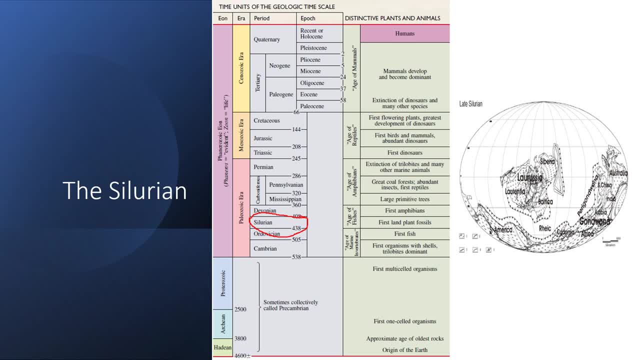 shortest Paleozoic period, spanning 24.6 million years. In the Silurian oceans, the Geode and Bonk fishes dominated in, dominated clearly in clearly diversification. 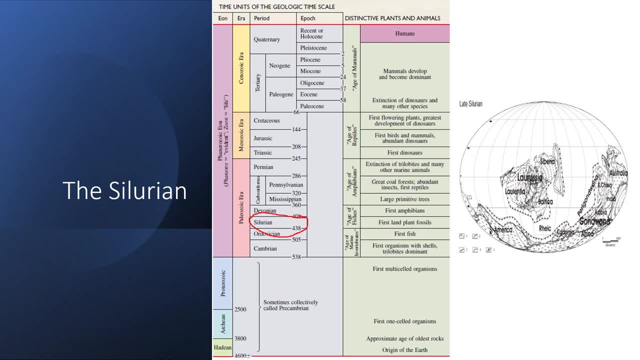 of the multi-cell life form, The Silurian system, distinguished in fossils bathing in sedimentary rocks in south worlds. The name Silurian come from one of the Celtic. 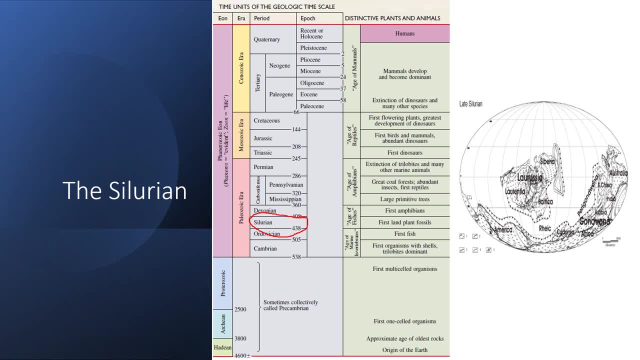 tribes of worlds In Bohemia, which is a part of Czech Republic nowadays, the Silurian system shows up in eight different stages, Which which points out the changing. 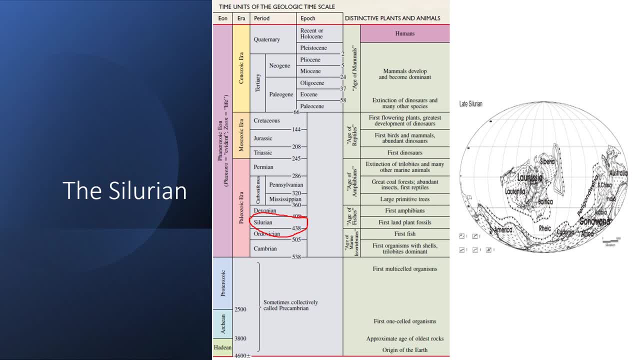 in the climatic events of the Silurian period, Which remarked also up to eight events of catastrophes happened in this period of earth history In the 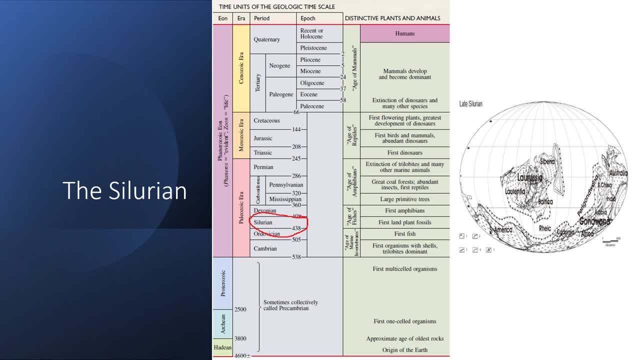 middle Silurian appears that 80% of continents extinct. This extinction event made the early vacant event of the middle Silurian The other markable. 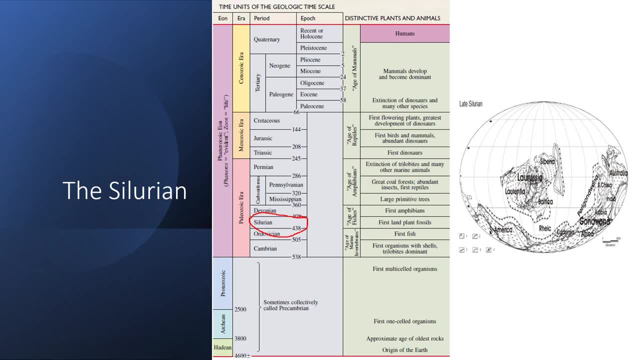 event named the Mold event, where oceans are toxic, with a lake of oxygen and rich in sulfur and sulfur gases of today. atmosphere of the. 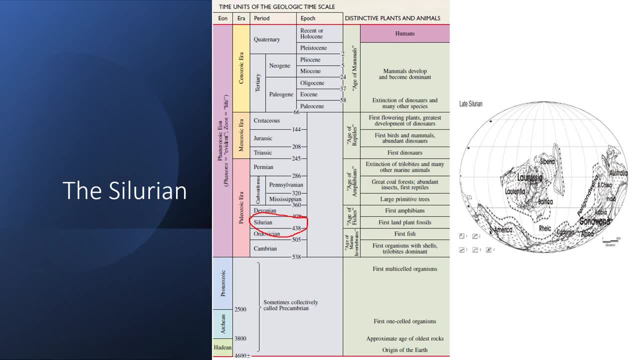 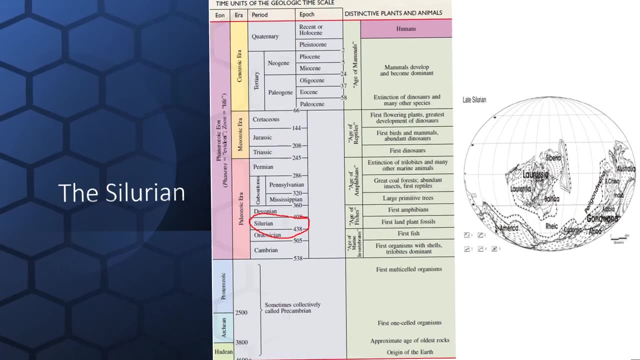 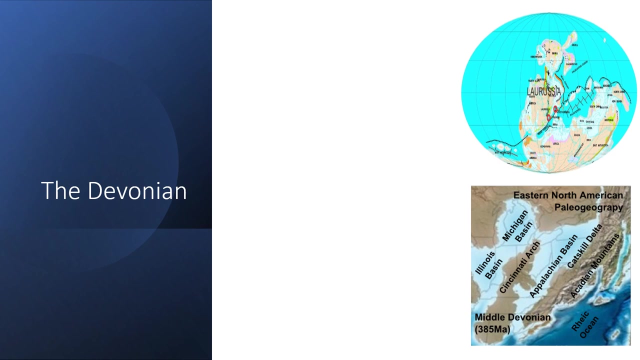 Silurian, The sea level dropped down globally and the toxic in Gotland, which is near to the Sweden. During the Devonian period, the Earth 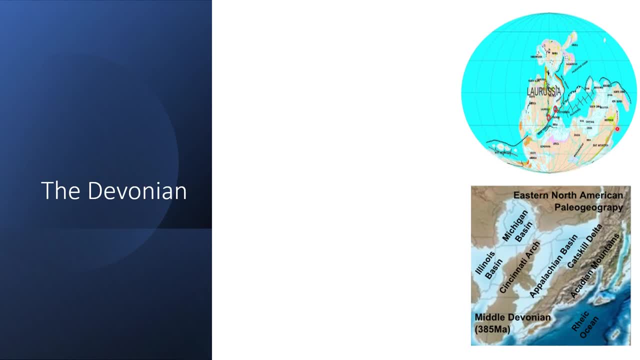 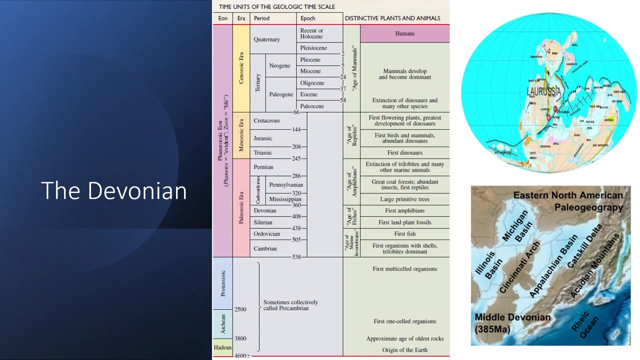 shows up in a paleo geographical map shown here, a mountain chains building processes of the Appalachian and Acadian in the North America. Regarding the 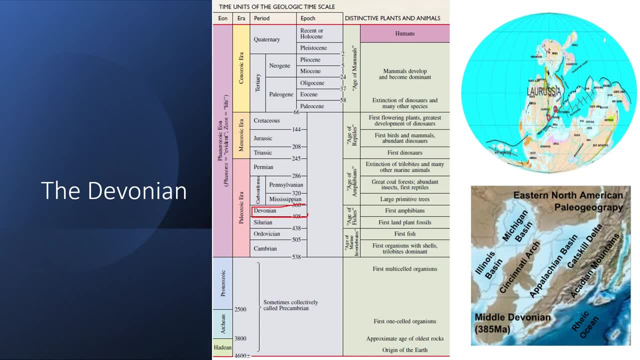 position of the Devonian. in the geological time scale, the Devonian position is: Devonia is an area named in England where the Devonian rock 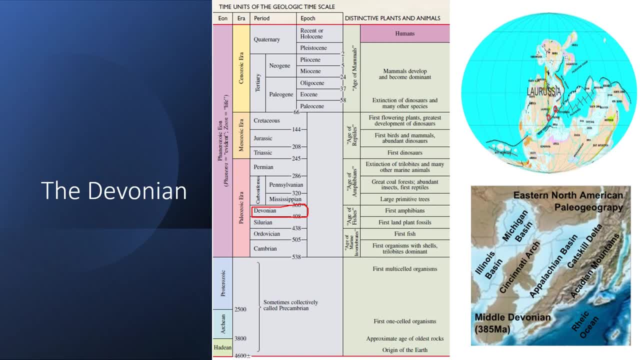 system from this period of history of Earth, history discovered at the first time During the Devonian life forms, the continents of the Devonian Fish. 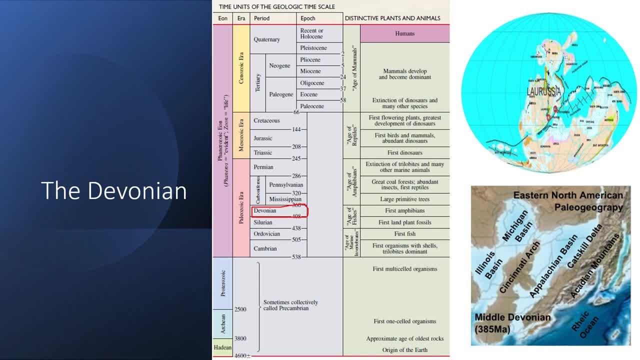 species dominated in remarkable diversity, and therefore the Devonian named the age of fishes The first mollusks, especially the, especially the ammonite, the, and. 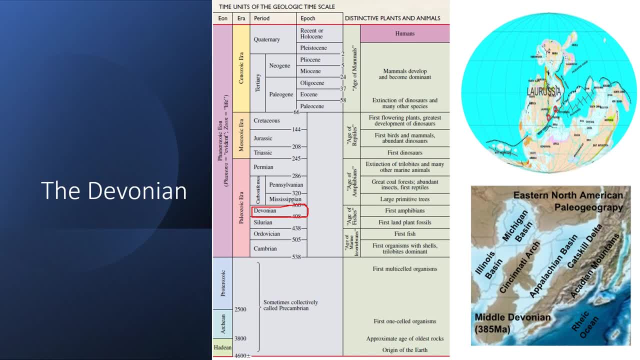 coral reefs appeared near to the shorelines of the Devonian seas. The paleo geography of the Devonian represented the super, represented by the super. 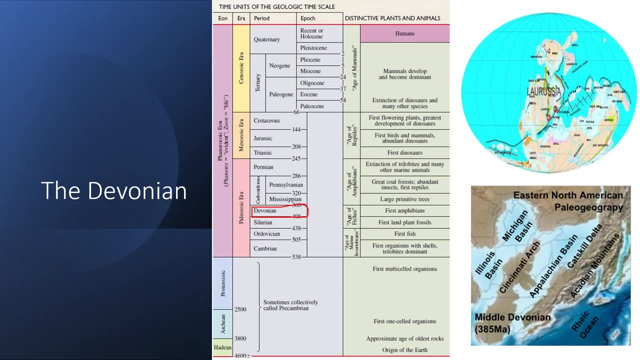 continent Gondwana in south, in south of the planet Earth, And the new continent Euro-America was in between these two great continents, The 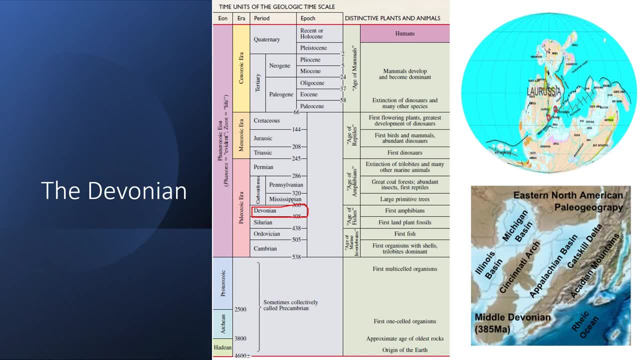 late Devonian marked with extinction, event which ended the Devonian period. The period was relatively warm. in the early Devonian the average sea water temperature 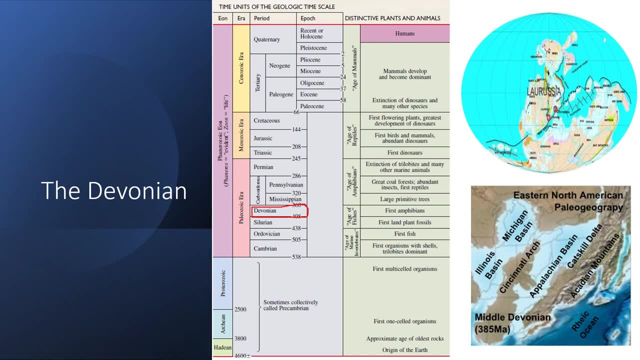 were about 30, degrees centigrade The. these temperatures recorded from an organism called the Gondwana and which changes in the sea water temperatures. 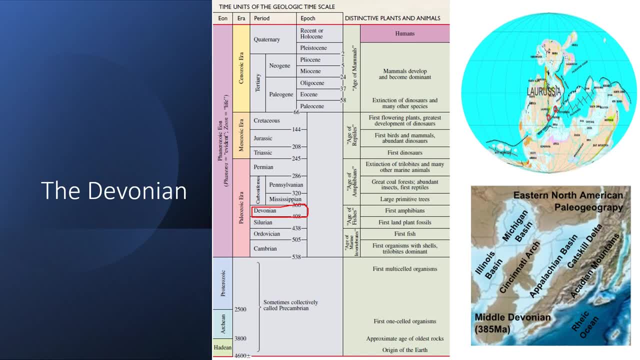 While the Earth equator areas was were dominated by the desert and dry land Because of the dropping in carbon dioxide concentration level. flora, the 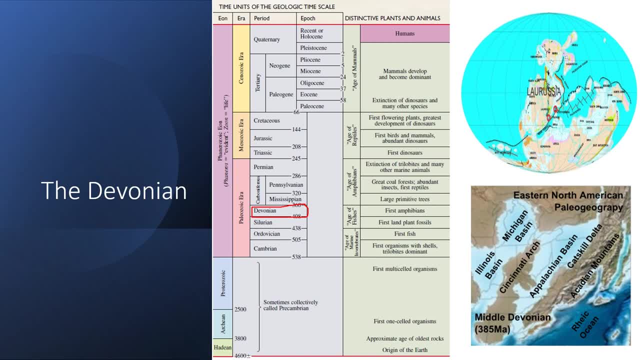 covered the covered and dominated the Devonian continental surface. These event made the made the global average of temperatures of the Devonian drop from 30,. 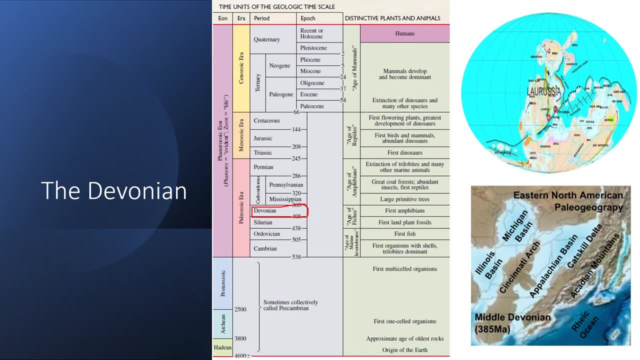 degrees to 25, degrees Increased in the continental surfaces and case the deposition and precipitation of the geological materials at the seas of the Devonian. 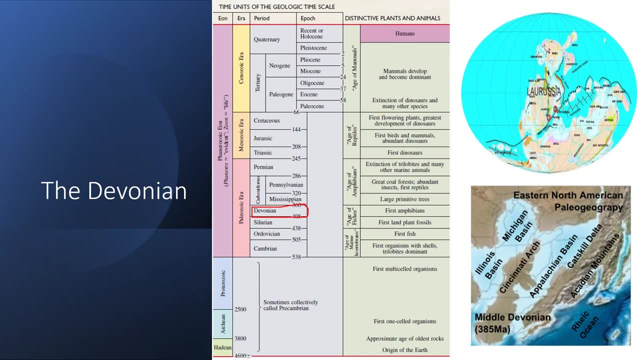 Casing huge and unbalanced load activities at the oceans floor. The Devonian, separated from the carboniferous by extinction event, spent around 30, million. 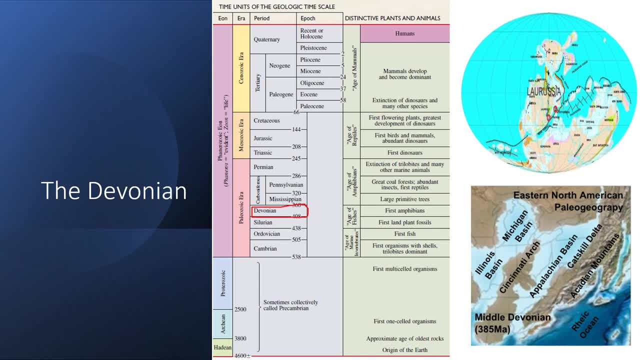 years. This event is known as the Hengeberg event or Hengeberg glaciation event: change in the global temperatures and, during this event, destruction. 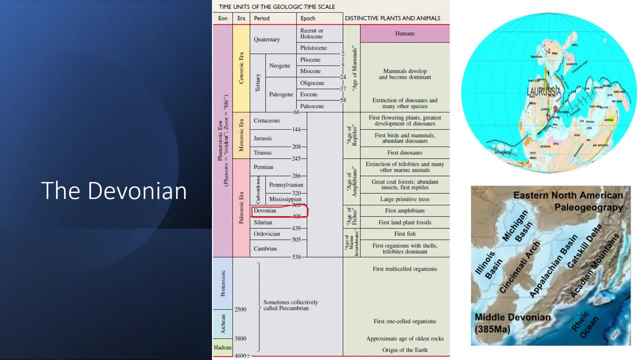 of the fauna and flora happened to the life forms of the Devonian period: The toxic. a toxic event also with the glaciation event. The earth. 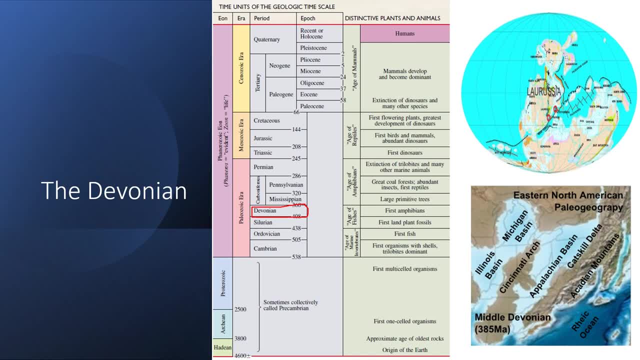 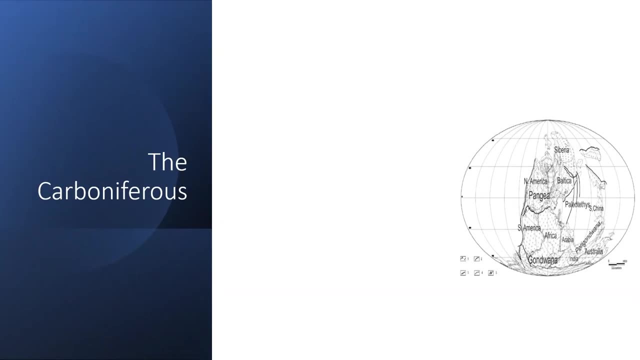 atmosphere was toxic and oxygen found dissolved in ocean water. all The carboniferous period and the paleogeography of the carboniferous is shown here. 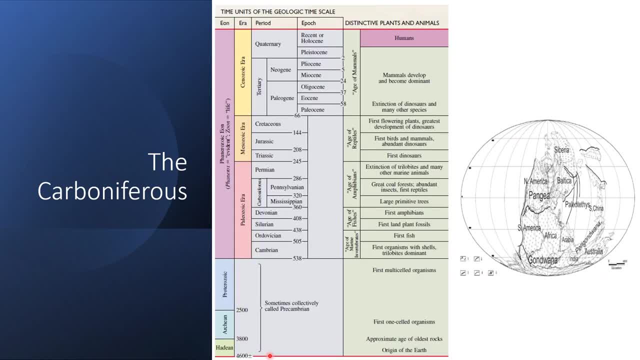 in this image. The position of the carboniferous period is shown here in the geological time scale and it is in the upper part of 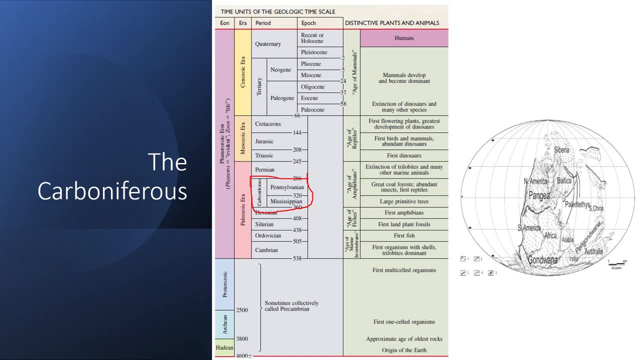 the region of the ocean and of the region of the ocean, The positions in the geological time and age of the ocean. All this was 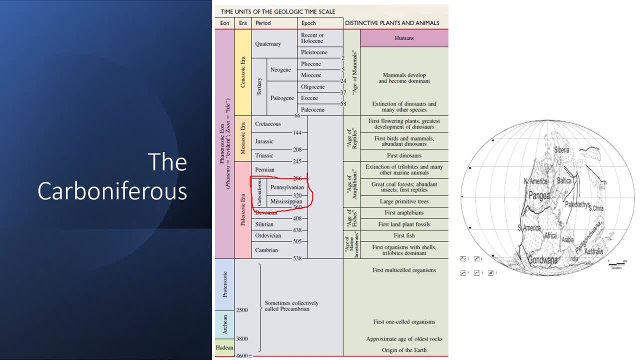 the position of the, the continental land and diversified to many lizard species, as snakes and crocodiles In the late Carboniferous or the Pennsylvanian. insects dominated the forest of the period and, in different species. Forests with different plants and tree types cover the 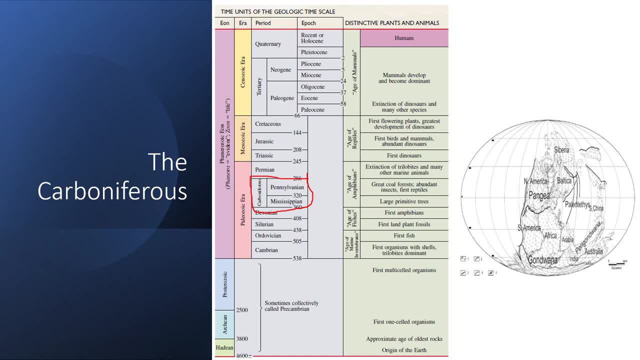 continents of the Carboniferous period. These plants cover become the source of coal that characterized this period of time. from the beginning of the Carboniferous period, the earth history, there are evidence shows that in the late Carboniferous oxygen gas, oxygen gas levels in the atmosphere was higher and up to 35 percent. 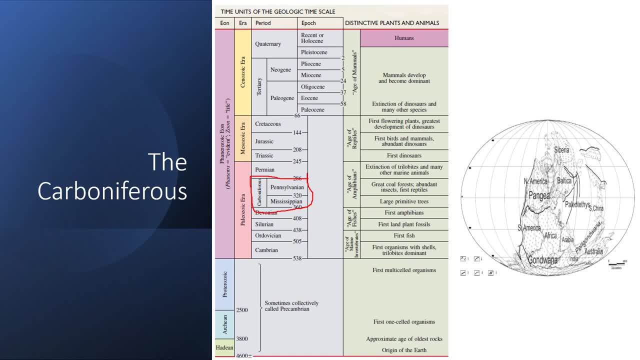 comparing to our day's oxygen level, which is measured to be 21 percent. the climate in the Carboniferous changed by a global sea level dropping down due to originies of the mountain chain, building processes and due to the continental drifts and continental collisions, and as a result of the 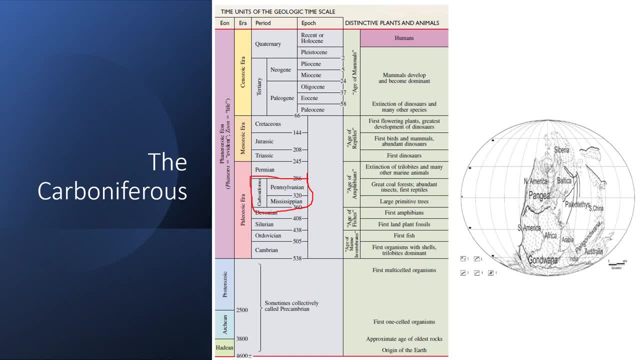 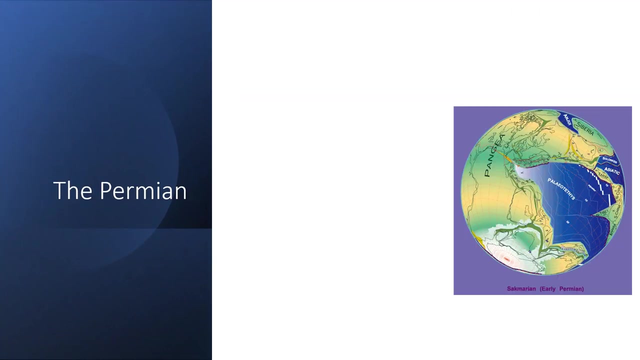 of this origin is the continent Pangea appeared on the surface of the planet Earth. The upper late Carboniferous, characterized by glaciation age, covered almost the planet, causing a total collapse to the rain forests of the late Carboniferous. The Permian, and the paleogeography of the Permian shows here in this image. 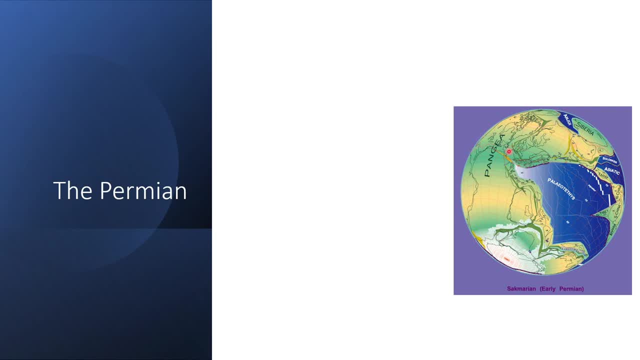 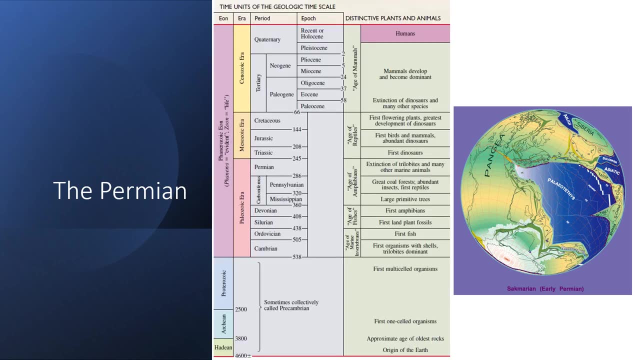 where the Permian or the Permian is associated with the region and it is the continent, Pangea, dominating the earth continents and earth surface. The position of the Permian is the upper part of the Paleozoic era and the name Permian refers to the Perm. 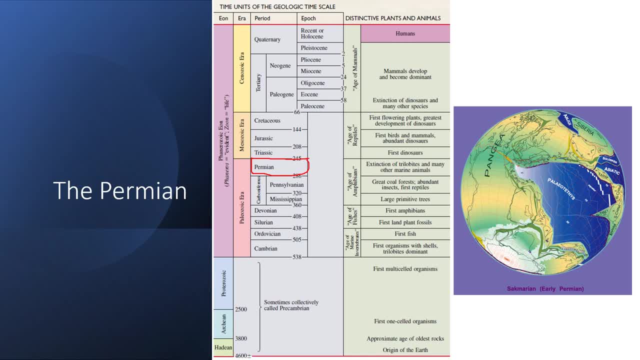 region of Oral Mountains in Russia. The Permian period, separated from the Carboniferous by ending of the Global Glaciation Age, started in the Carboniferous period. The Permian period characterized by the appearance of a great continent, Pangea, On the land. diversification of 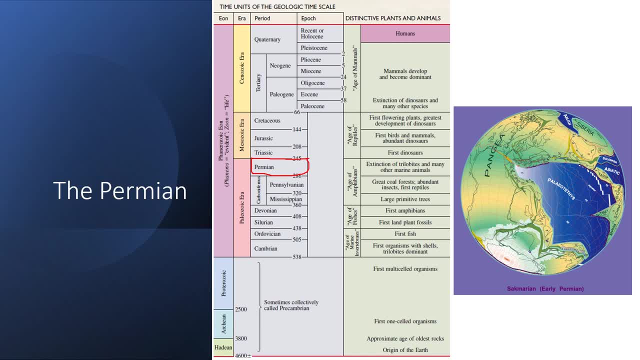 synopsis and reptiles were notable and noticed in rock formations belong to this period. The super continent Pangea formed from collision between Ura, America and Gondwana. continents Early in Carboniferous resulted in the in in the huge mountain change of 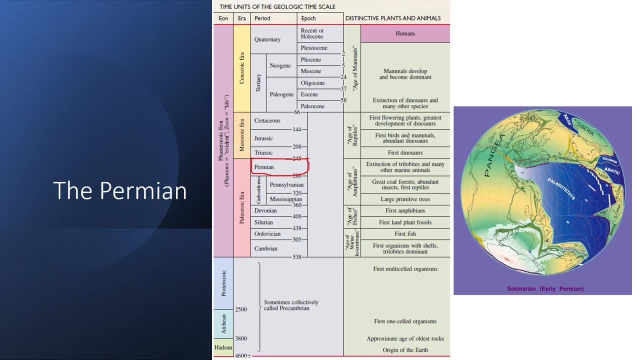 Hamalaya, which is up to eight kilometers from the sea level and at the edge of the social line of the collusion of these huge continents. the Pangea was surrounded by the the great oceans of Panthalasia. The major event of the Permian is the volcanic eruption of Emishhan. 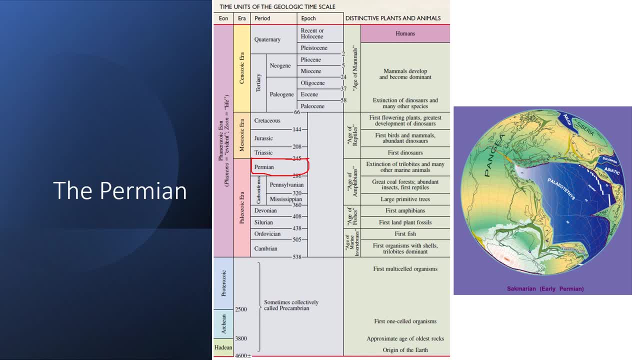 southwest of China and Siberia north of Russia. The volcanic events destroyed around 80 percent of the life forms covered配合 facade characters that 나타�ned, the Permaiont growth Prize, which is known as the originally deficient galactic development of the Pyramid, and engage in distress by the impact of erosive increase in forced evacuation to衝突nias. How is the water? affect Do the accidents in emiss存在 씨家 and the eastern constellations in Russia dissipating forces in only just a few weeks. MažBBĀ� About Re acquaintance from the E. количество proršechi education 감사. 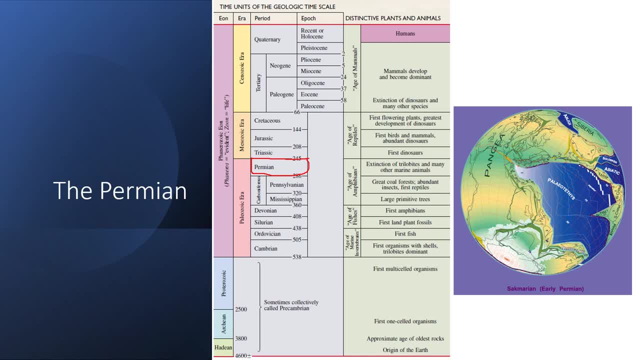 uita houla vabar Jungka чет bonds confidzone les animas opäksämcible. iya a'hráç hexği u p. trostia ve hulçâçămittă on the continental areas of the Permian and also 70% of the marine life forms also. 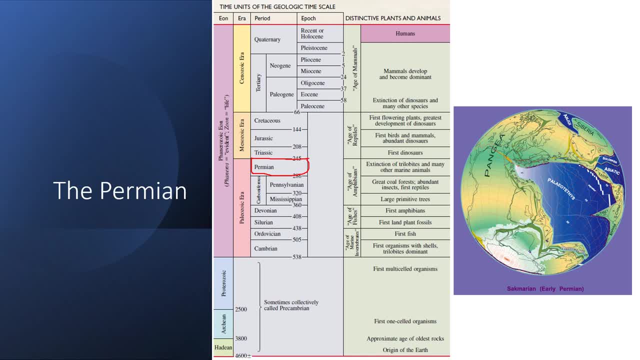 distinctive This event preserved in the rock formations belonging to the Permian period. The Permian atmosphere, temperatures were extremely variable and cased monsoon, rainfall, falls and descents- topography that dominated the Pangaea continent. The best Permian presentation of the Permian-descended formations showed up in Texas and New Mexico's red beds. 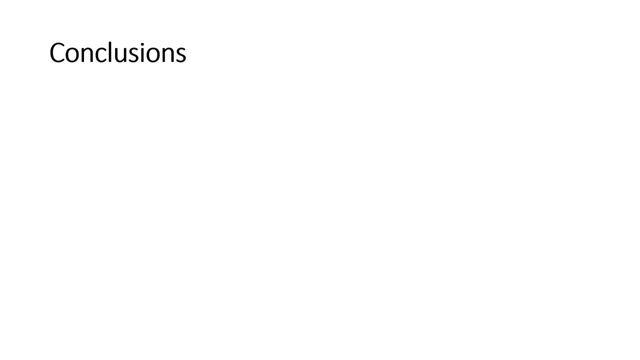 Now we have come to the conclusions of the presentation for today. The planet Earth in the lower part of the Phanerozoic Eon suffered by four major and global glaciations, turning the planet Earth into snowballs, destroying surface and marine life forms. and rose again in different shape and life forms and preserved oxygen concentration levels in the atmosphere. The planet Earth suffered from many continental drifts during the Paleozoic era, shaped and reshaped the continents through regional orogenies of mountain chain building at the suture line of the collided continents. 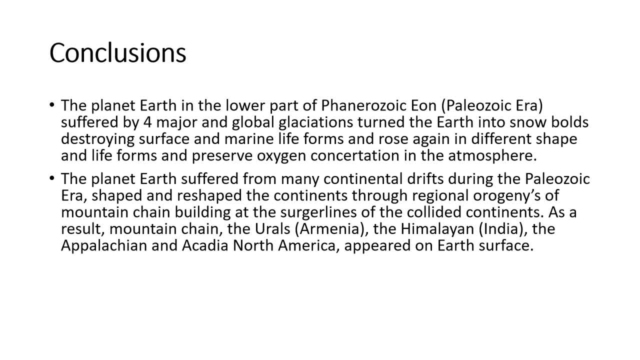 As a result, mountain chain, the Oral in Armenia, the Himalayan in India, the Appalachian, the Akkadian in North America- appeared on the Earth's surface. Almost 28 climatic shifts and changes recorded during the Paleozoic era due to meteoroids, impact and global volcanic eruptions. 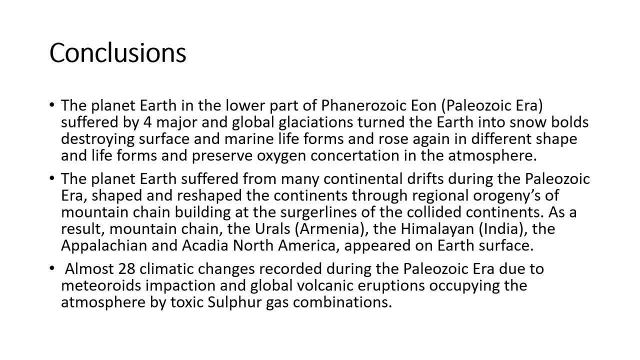 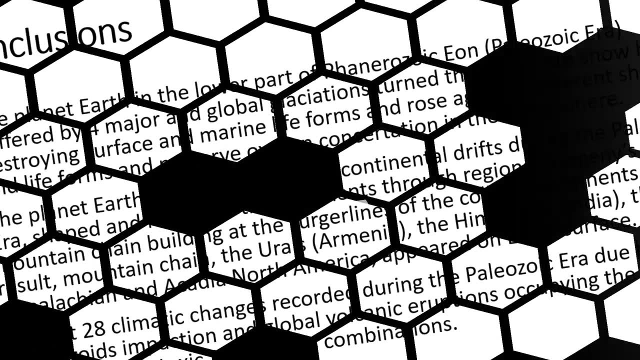 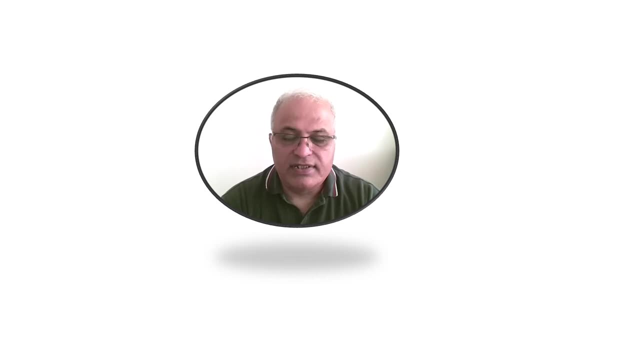 occupying the atmosphere of this era by toxic sulfur gases combinations. As a result of these changes, the temperature of the ocean was reduced, and the temperature of the ocean was reduced. This is the result of these changes. Thank you for watching this presentation. My name is Sabah.